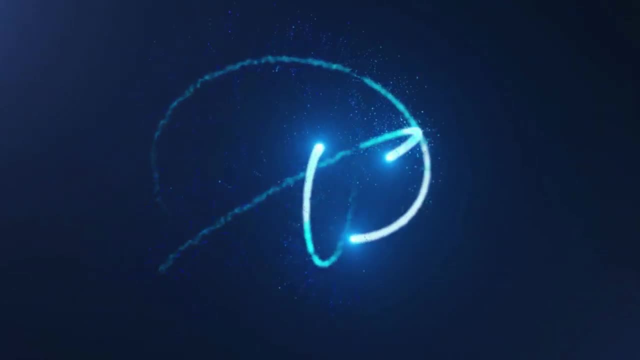 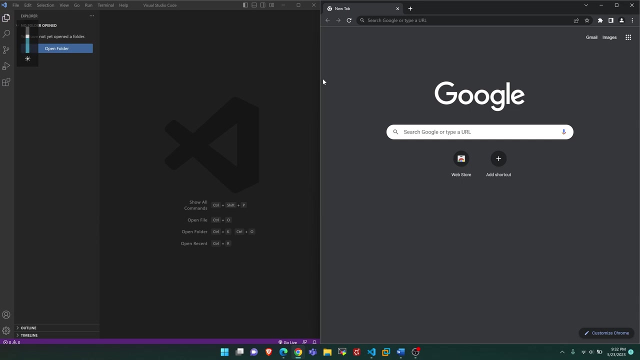 Hello again as pairing coders, Welcome back to javascript for beginners. In this episode we will learn about operators, control structures and functions, So let's dive right in. First, let's set up the environment, As we have used chrome console in the previous episode. 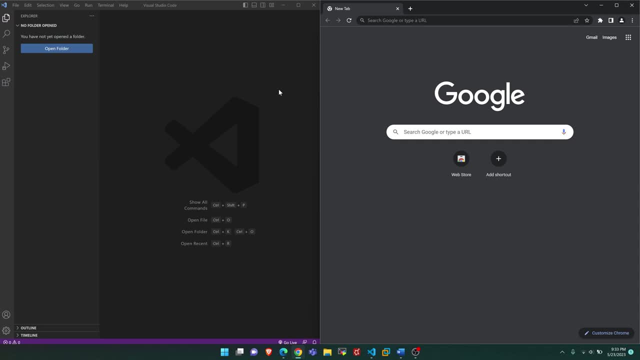 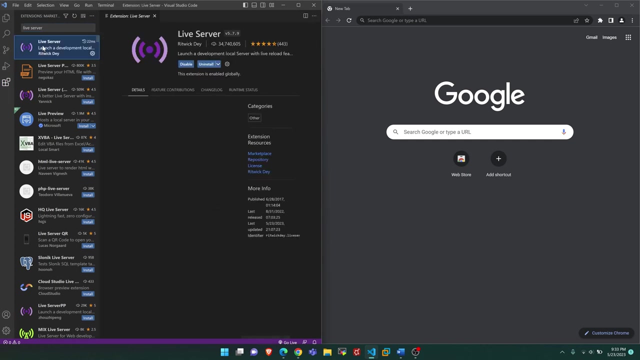 today we are going to be using directly inside the vs code. So in order to do that, we will install an extension called live server. For that, head over to the extensions tab and then search for live server. As you can see, I have already installed it. You just have to press install over here. There will. 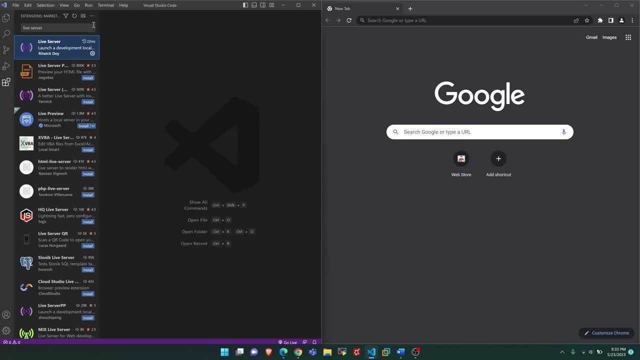 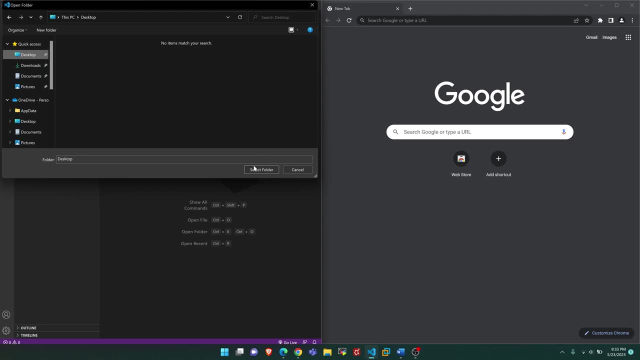 be a button over here. Once that's installed, let's open the folder where you want to develop. So I will open my folder as desktop and then head over there and then select the folder. So once you have that, we will create an indexhtml file. I already have one. I will delete it. 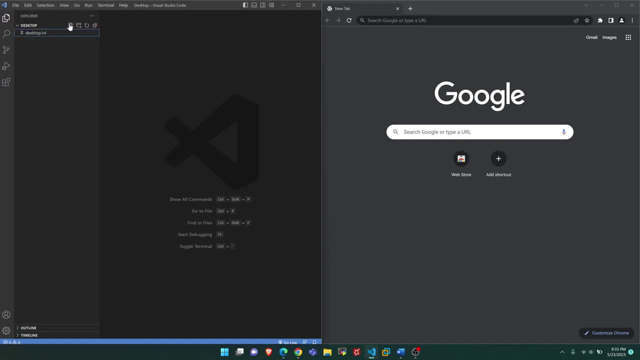 and then I will create an indexhtml file over here. Then just press the exclamation mark. It will. it will give you emit abbreviation which is inbuilt by vs code itself. So you just press enter, which will give you an html boilerplate. So 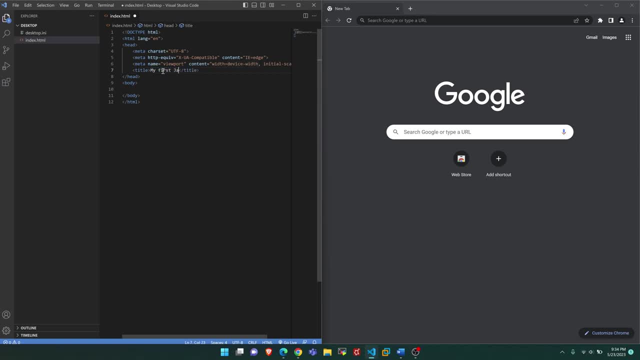 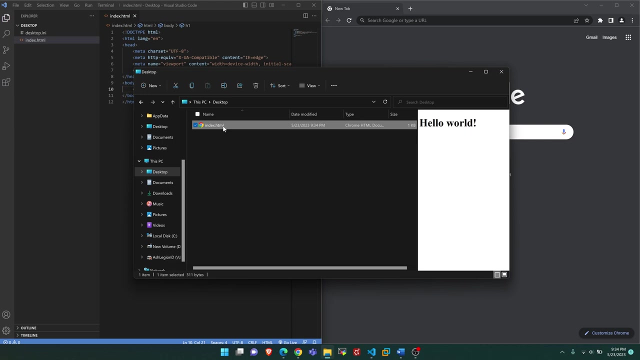 right now I have one. I will rename the title to my first javascript code and then I will give an h1 tag saying that: hello world. So once you save it you can open that in the chrome browser. So for that I will head over to my desktop and then I will double click on indexhtml. 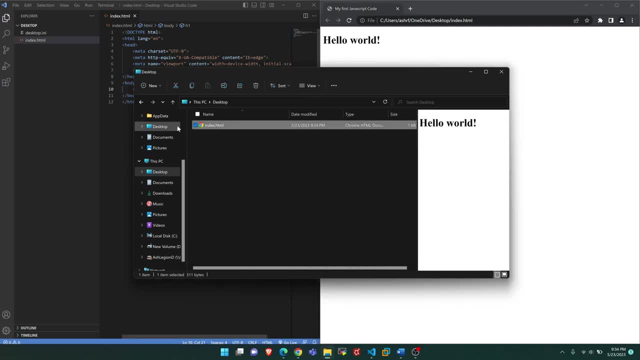 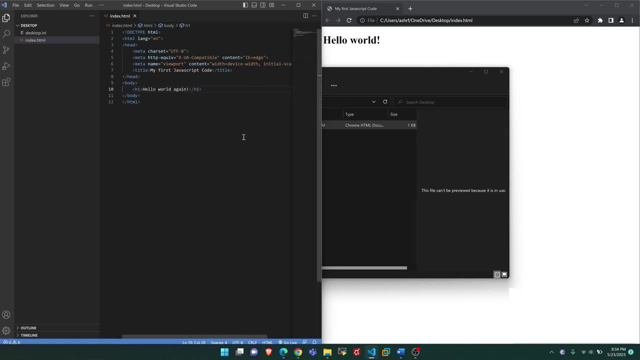 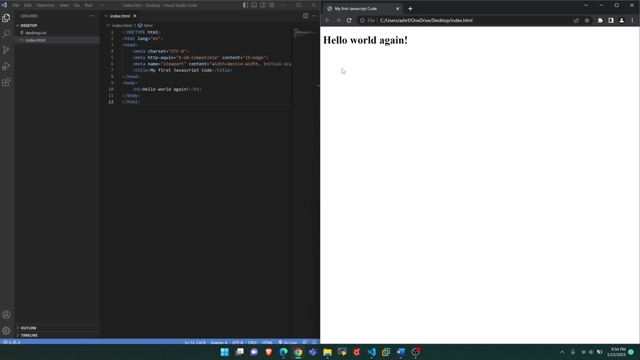 So this will open my hello world. application with this approach is that whenever you make a change, you have to go again to the browser and then refresh again, right, so this is not feasible all the time. so, as a next step, what we will do is we already have live server installed over here, so this is the live server. 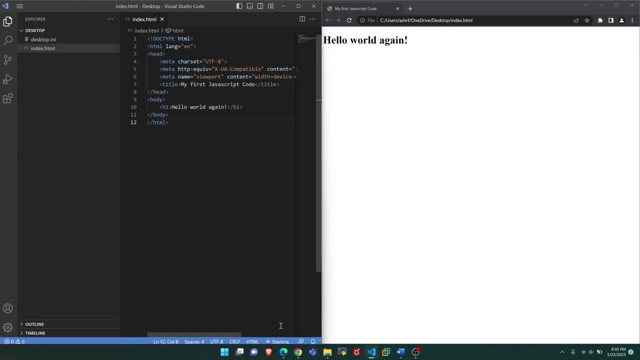 so you just press on click to run live server over here, which will automatically start in a port and then it will automatically open in the browser itself. so let's say you have made a change and then press saved to automatically refresh for you. so now that the environment is set up, 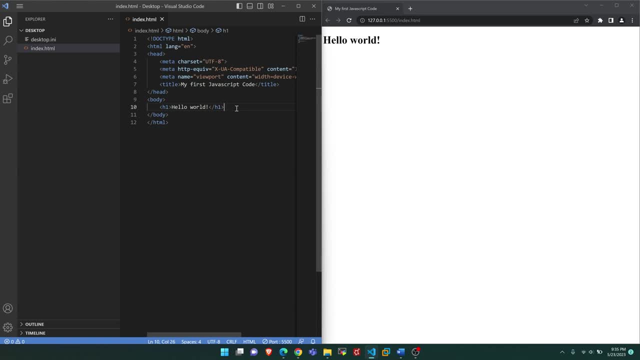 let's dive into the concepts of operators, um functions and console structures. so to write a java script code, we will. we will have to create a script tag inside the body. so we'll create a script app and then just to see if it's working or not, we will just put consolelog. 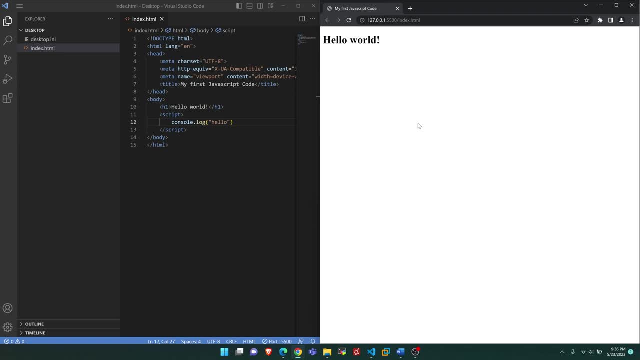 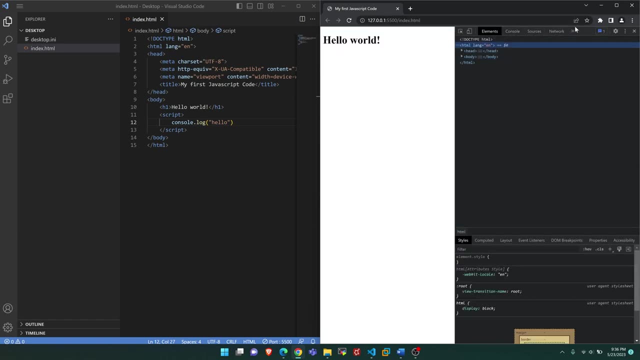 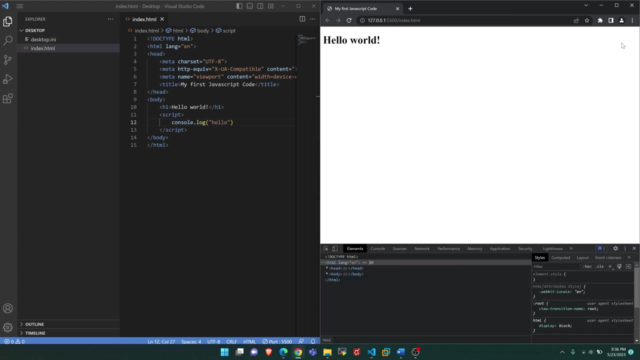 hello and then you save. let's check if it's working or not. so, for the same way, click on inspect. it will open up with the console. for the sake of viewability, i will put it in the video bottom part of the Chrome and I will increase the width and then go to. 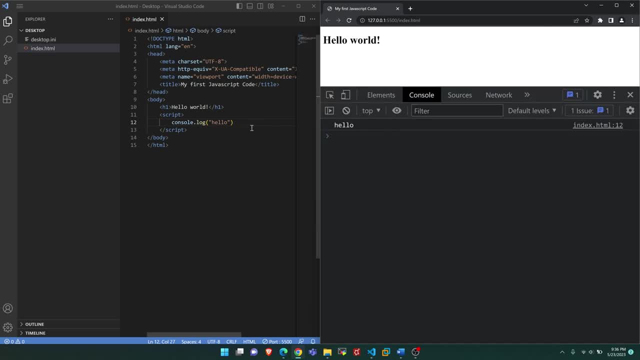 console. as you can see, it's already there, so that part is working. so now the next step will be learning about the operators. so in JavaScript we have several types of operators, including arithmetic, assignment, comparison, excuse me, so basically we have arithmetic assignment, comparison, logical and others. so some of the example can be, let's say that, a equal to 10 and then 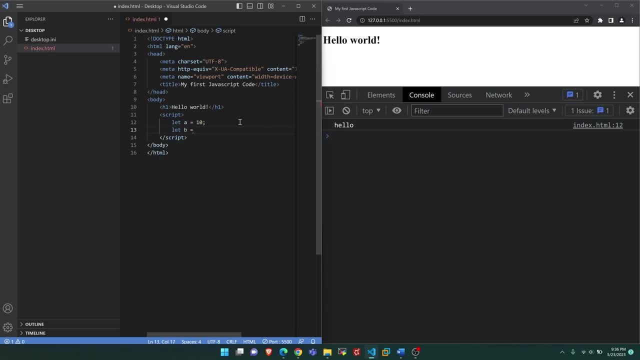 let B equal to 20. so this particular equal operator- we can call it as a same and operator- we are basically assigning a value of 20 to B. now if you go ahead and try, like simple basic automatic operations, you can see that the number of operations is increasing and then the 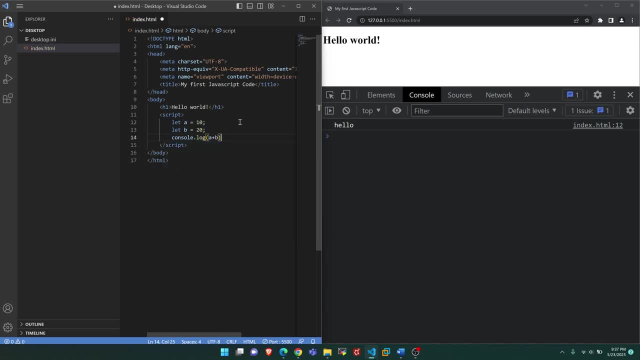 the number of operations is increasing, and then the consolelog it will give you some answer and then if you do a minus B, and then you can also do a divided by B and then in also do a star B. so, as you can see, the value we are getting is like a plus b, it's 30, correct, and then a minus B is. 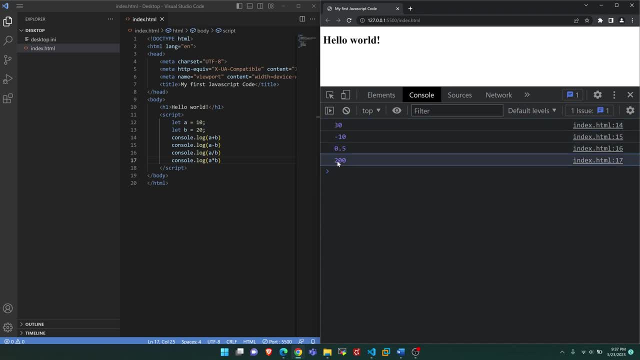 ten, 10 by 20 is 0.5, and then 10 into 20 is 200. so these are the arithmetic operations that we have at hand in javascript. so that's as simple as to explain how the arithmetic operators work. now let's move on to the console control structures. control structures help us control. 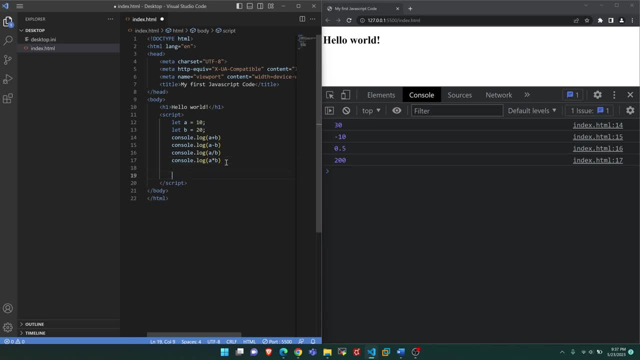 the flow of our program. the most basic control structure is if condition. so let's say we have a equal to 10, right, so we will create another variable correlate number equal to 5, and then we can write a simple if statement as if opening bracket number greater than 0. 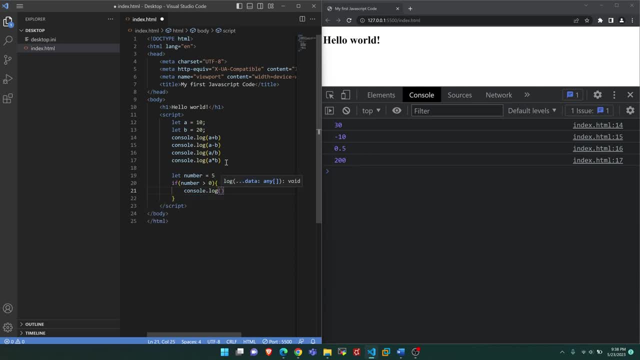 then print. for now we will consolelog: uh, i am. i am a positive number, right f, not. in the else part i will say consolelog, i am not a positive number. so, as you can see this code executed and we are getting, i'm a positive number, let's say we change the value to negative one. 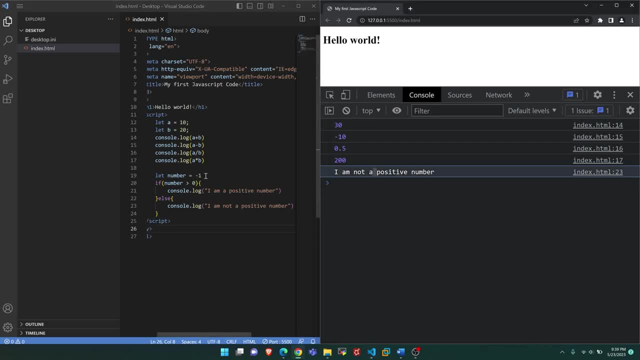 so we can. we are getting- i am not a positive number right- so that's the most basic uh control structure as we have. there are so many other control structures, such as switch, and then some other things are there. uh, we will go into detail of each of them. 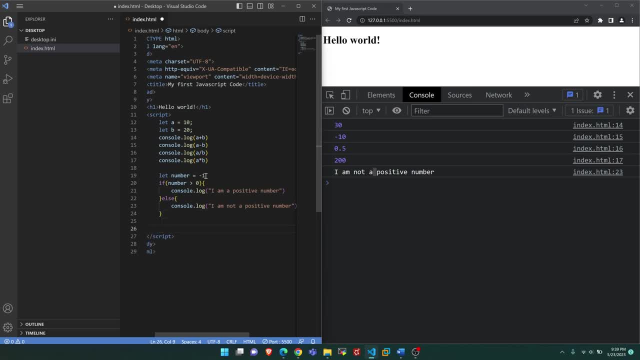 in the advanced javascript classes. now, uh, let's discuss functions. what are functions? so these are just basic concepts. i'm just like swimming through it. uh, later on we will use all of these in detail. so functions are reusable blocks of code that perform a particular task. so a simple example of function that adds two numbers: we can create it here itself. 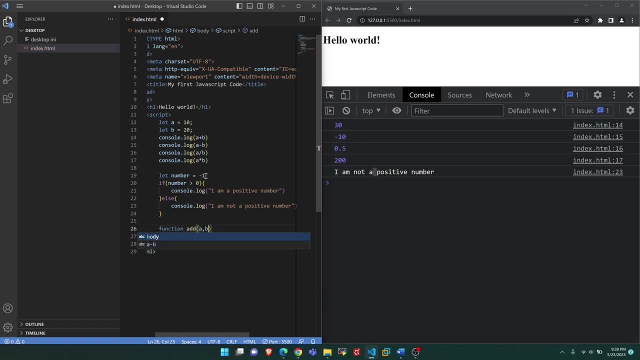 so let's say: function add, and then we will accept two values, a and then b- let's name it like that for now- and then what we will do is return a plus b. so what it does is it will take two parameters and then add those parameters and then return it back. so how can we do that? how can we call?